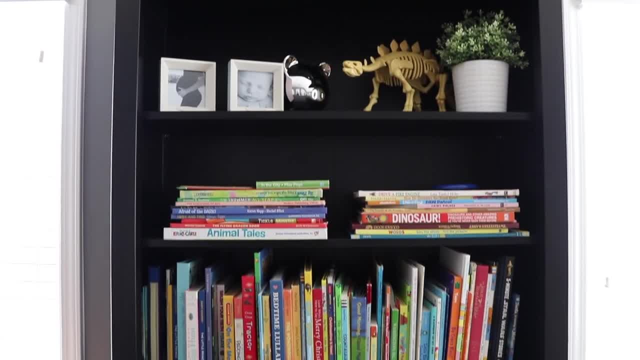 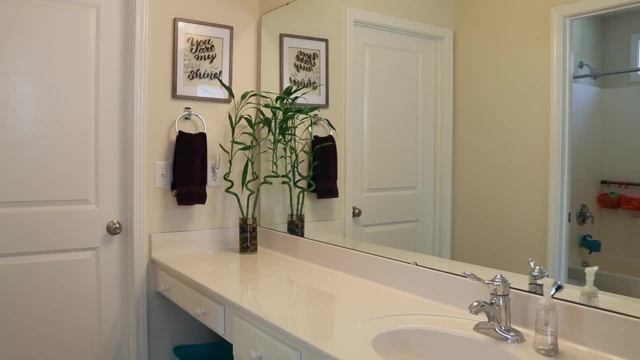 Now if you have seen my room tour video of Carson's room, you know that I love cheap things, thrifted things, everything is from the dollar store, because I'm pretty sure that phrase- this is why we can't have nice things. my family invented that There's no need to spend a lot of 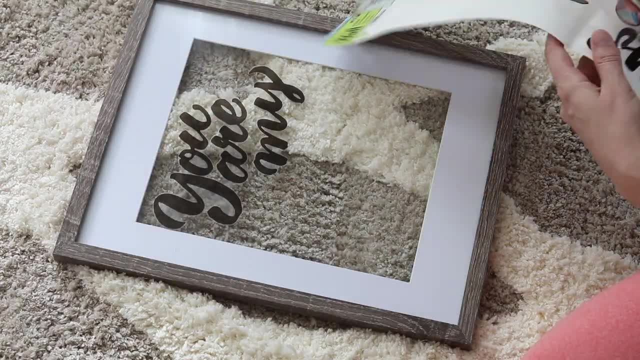 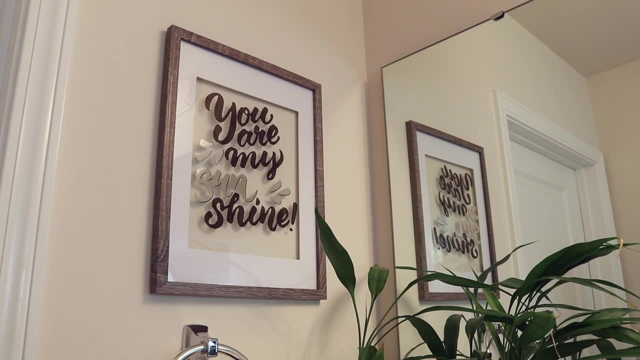 money on kids' stuff Rather than spending $20, $30 on a Hobby Lobby type frame. I went to the Dollar Tree, got a $1 decal, stuck it onto a frame I already had. It's beautiful and super cheap. 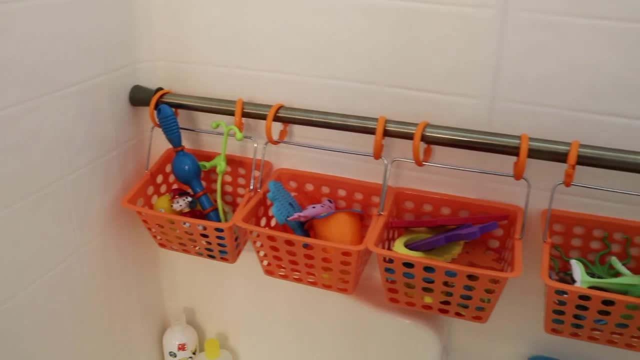 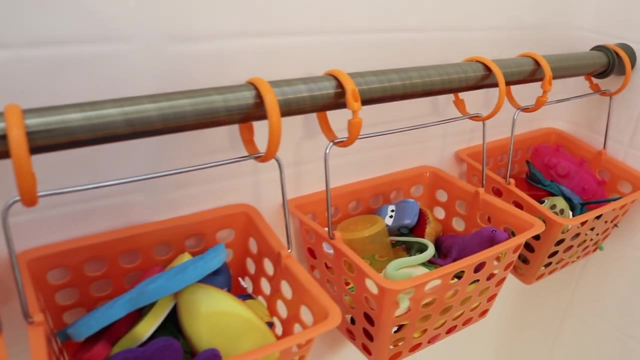 So let's start with how to organize your bath toys. All this is is a shower curtain rod, dollar store baskets and dollar store shower curtain rings. This is an excellent way to dry toys after you play with them in the tub, And I would say, as far as 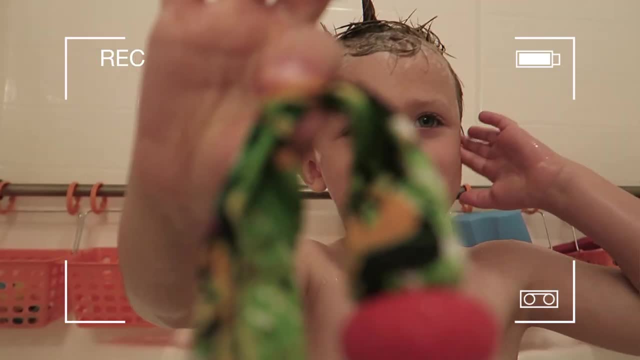 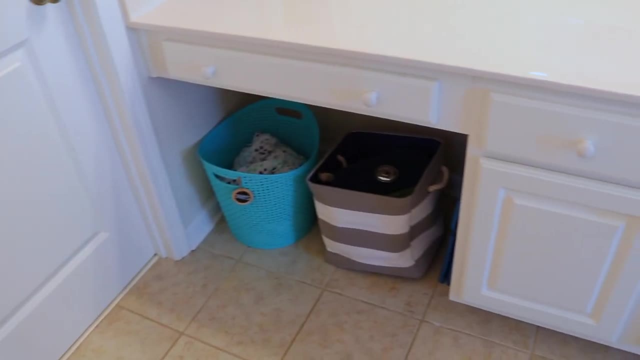 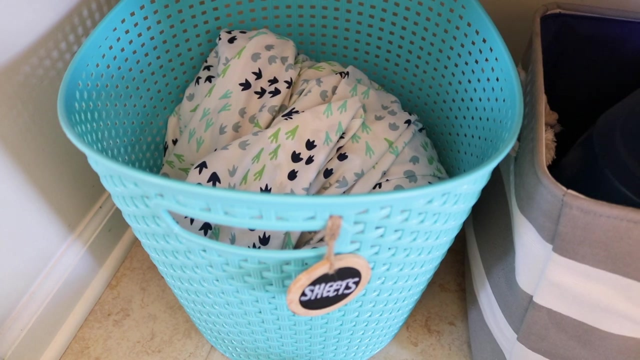 kids go, it stays pretty organized. That's why it's his favorite toy. This is a Jack and Jill bathroom, so it connects the boys' rooms, And underneath this open space is where I keep extra sheets, the humidifier and the stool. Why keep that in the linen closet when 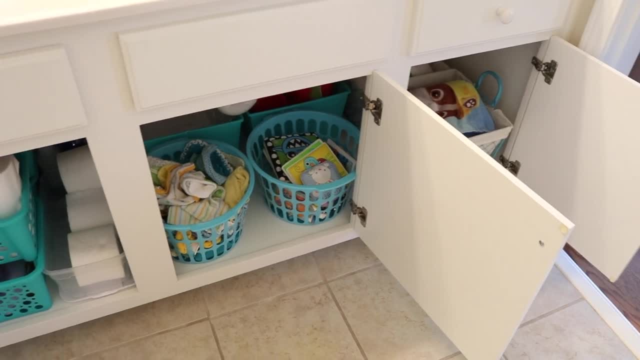 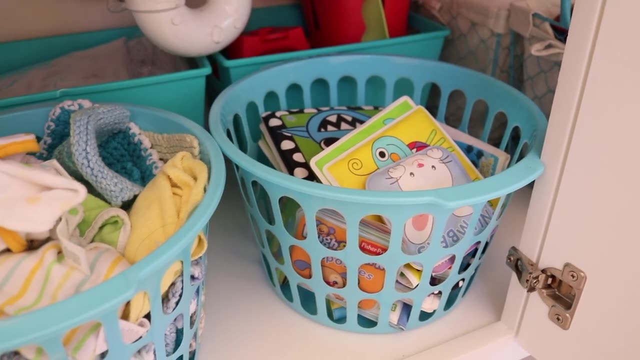 this is the spot I need to access it. Put stuff where you use it. All of these are Dollar Tree bins. I've stacked up toilet paper, extra soaps. I also have a lot of stuff that I can use to keep the boys' washcloth in here and extra bath toys that we rotate out, And I keep their towels. 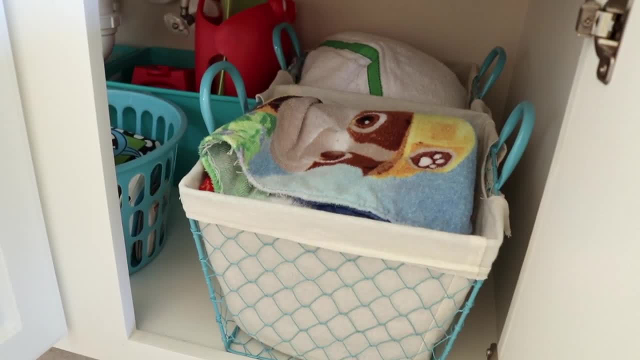 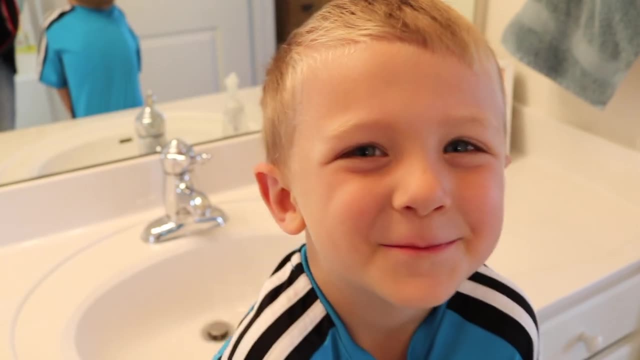 right in the bathroom. Again, why keep them across the house? You want to keep it convenient. I like to keep the drawers really simple. I've got Dollar Tree bins in here where I keep the toothbrushes, toothpaste. I also recommend all bathrooms have a sign to remind your kids what. 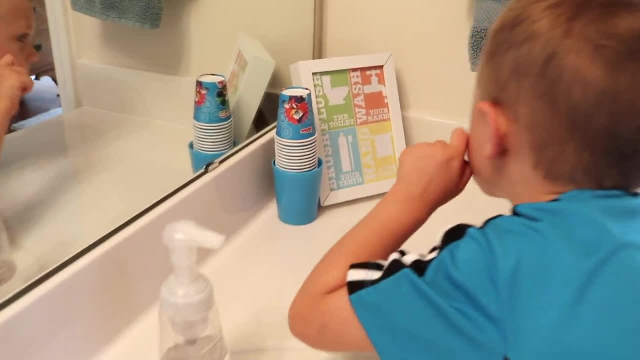 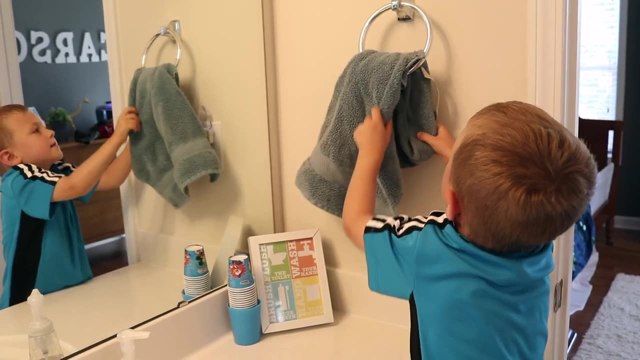 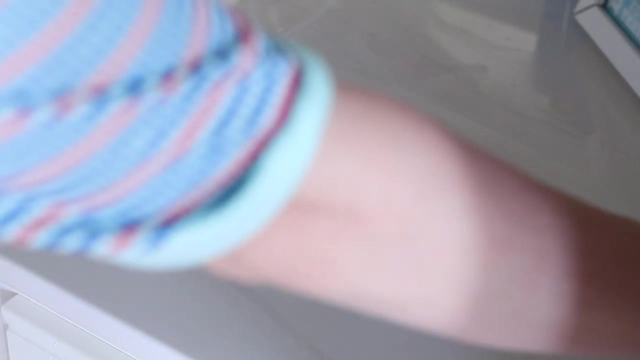 they need to do. This means flush the toilet and this means wash your hands, and this means toothbrush and toothpaste and this means towel- hang up towel. So here's how we keep everything clean. Once every day or so, I go through and I use one of my water. 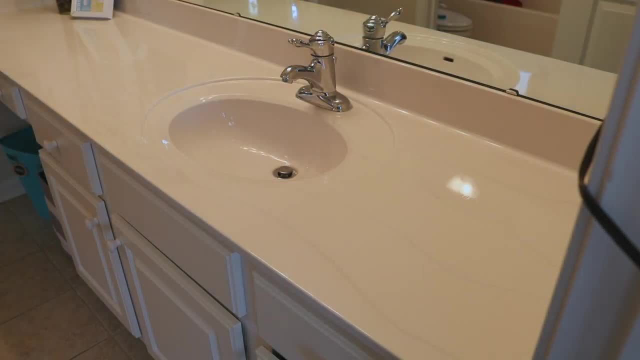 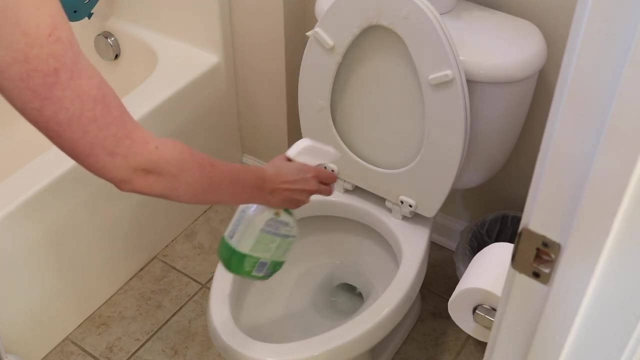 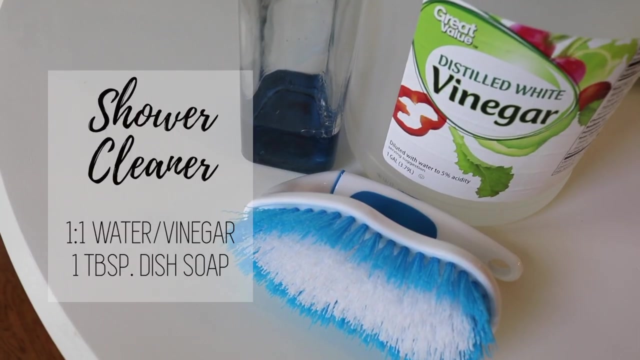 only cloths. I got these from eCloth to wipe down all of the countertops, To clean the bath and shower. I use vinegar, dish soap and soap. I use a lot of soap. I use a lot of soap. I use a lot of.